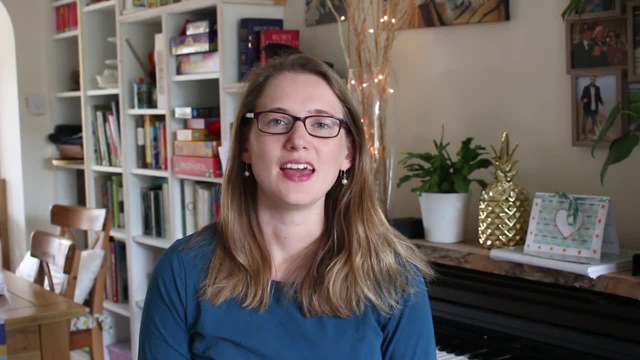 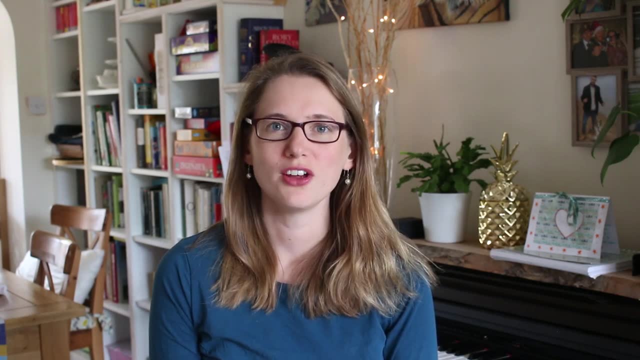 Hello and welcome to Starfish Maths. My name's Sarah and today I'm going to look at integrating using partial fractions. This video today is building on a whole series of integration videos that I've covered so far, so you can check out my playlist and watch basic integration reverse. 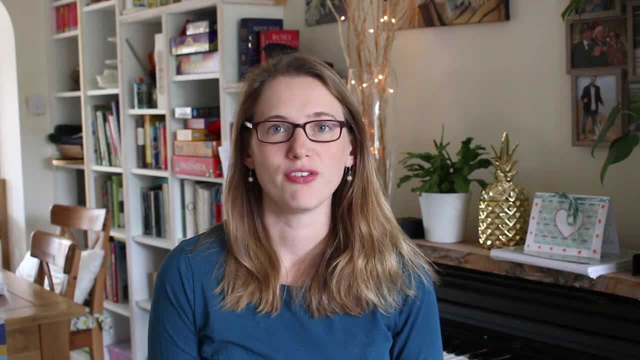 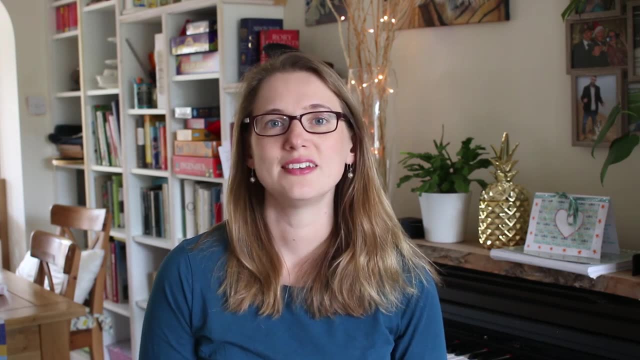 chain rule, integrating logs and also partial fractions. You're going to need to be able to do all of those topics before you can do the video today. So this topic today is bringing all of those things together. so make sure you've done lots of practicing first. I'm going to cover four. 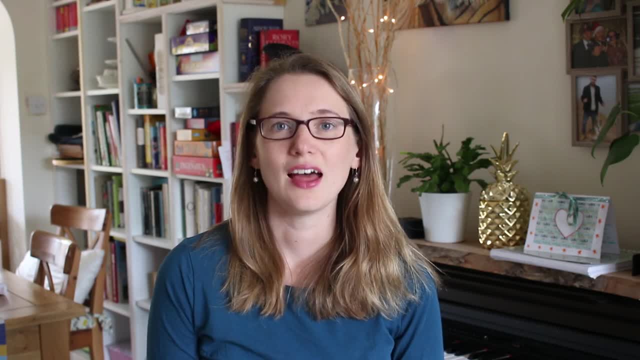 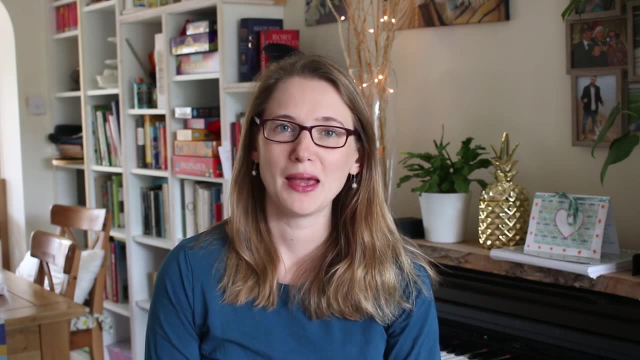 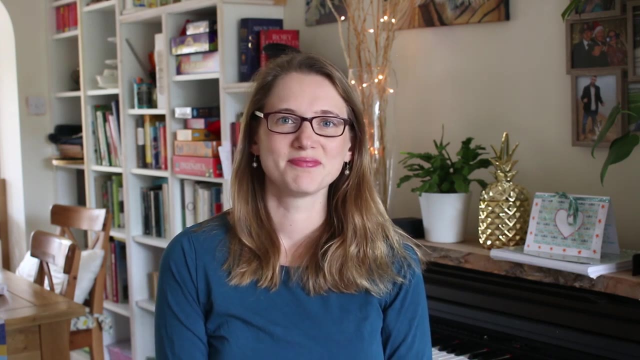 exam style questions- and the last one is particularly challenging- that I made up, so it's very hard, As ever. please do grab a pen and paper, pause the video and work at your own pace. I hope this is helpful. Let's get started. Okay, so here's our first question. So we're 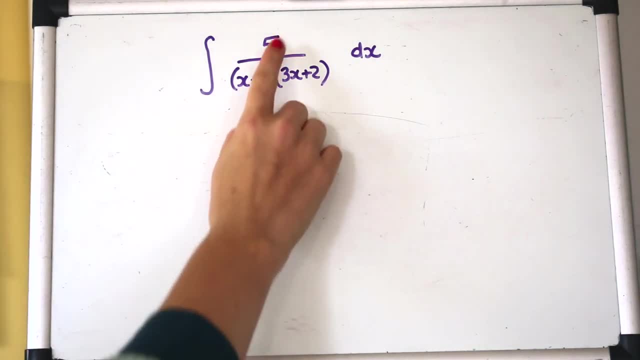 going to attempt to integrate functions that look like this: when you've got complex fractions and that looks like you can be split up. So we're going to use partial fractions before we integrate it. So, before we integrate, we're going to take this to the side and we're 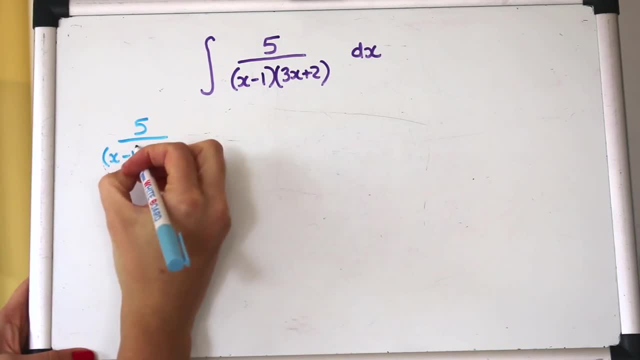 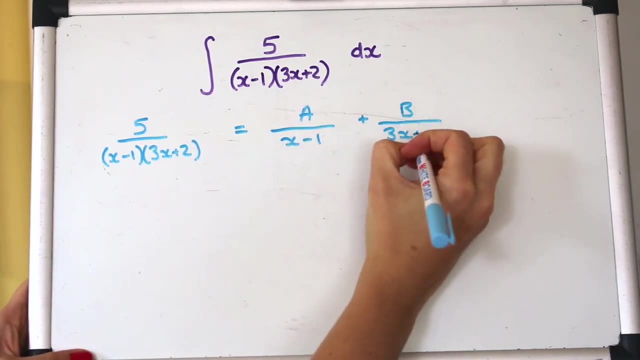 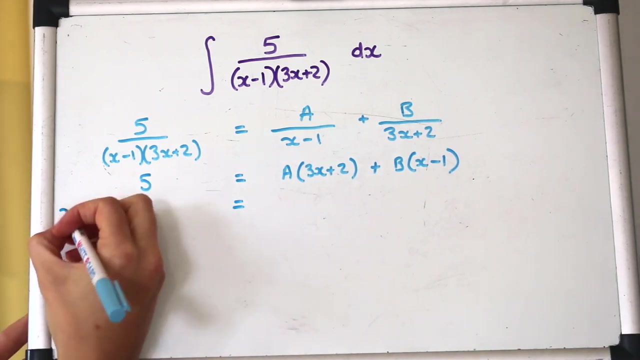 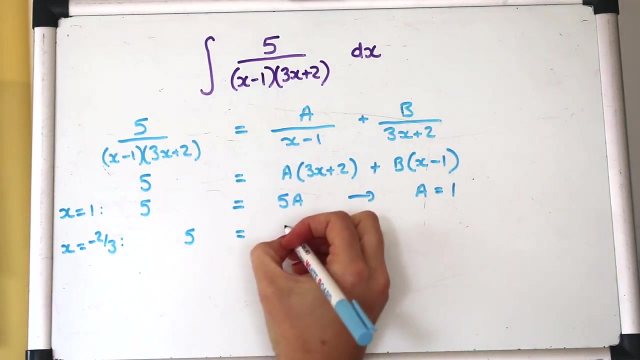 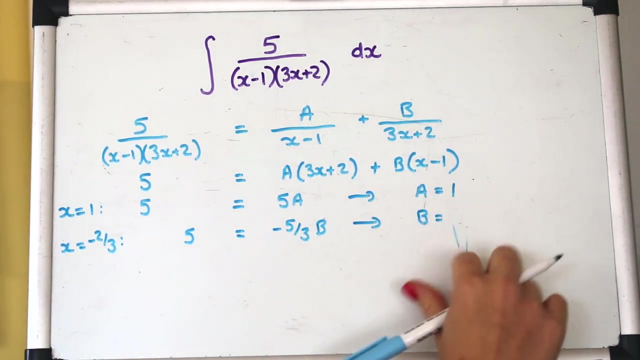 going to split it up. Hopefully you can do your partial fractions, so do pause the video and have a go at doing this yourself. I went through that pretty quickly, so do check out my other video on partial fractions if you need to brush up on that. 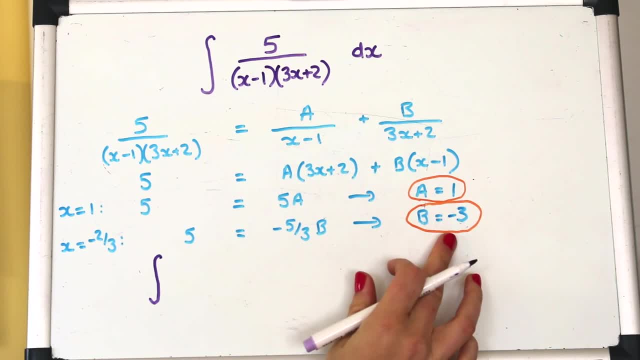 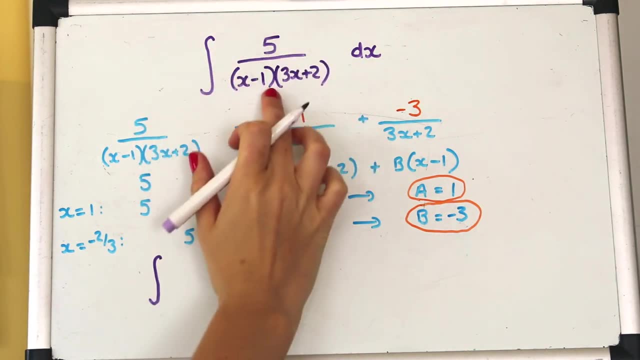 So now what we've done is we've expressed well, we found out a and b, so we can put them back. So now, instead of integrating that function as it stands in purple, we can integrate it as the split up partial fractions. So I'm just 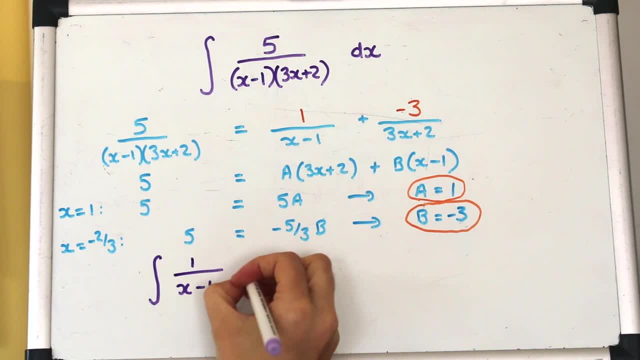 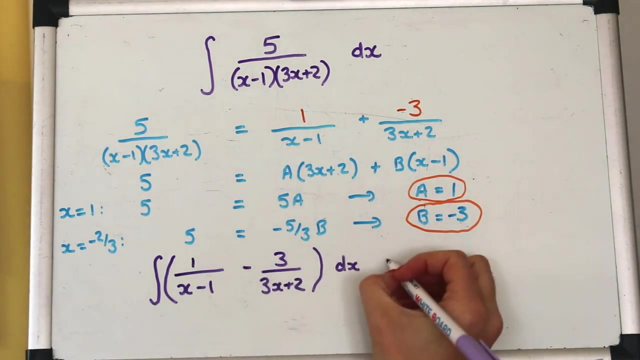 going to write out the integral with those partial fractions with minus three, like that. Of course we're integrating the whole thing, so it does need to go in brackets with the dx. We're staying here with an indefinite integration, so no limits here today And 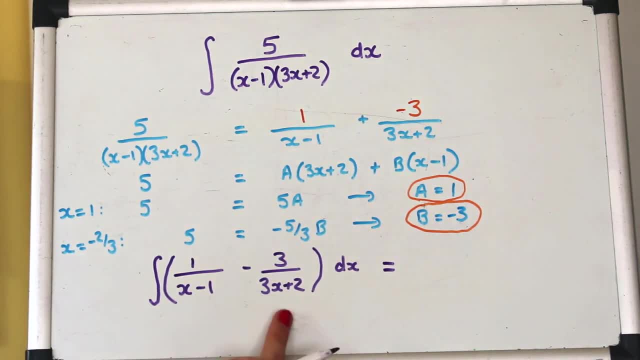 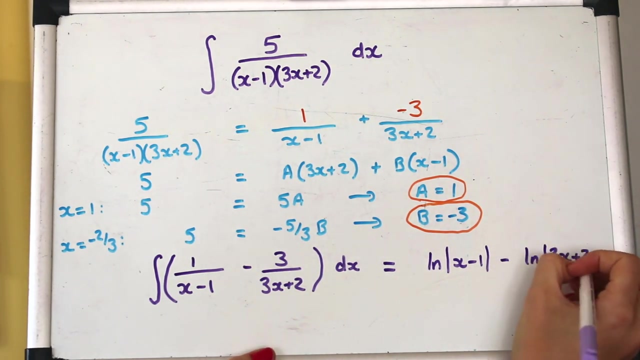 now hopefully you can see, because these are more simple fractions. you can see that I've got a very simple expression here. These are just straightforward log integrals, so that first one would be log of x minus one in modular signs and log of three x plus two. 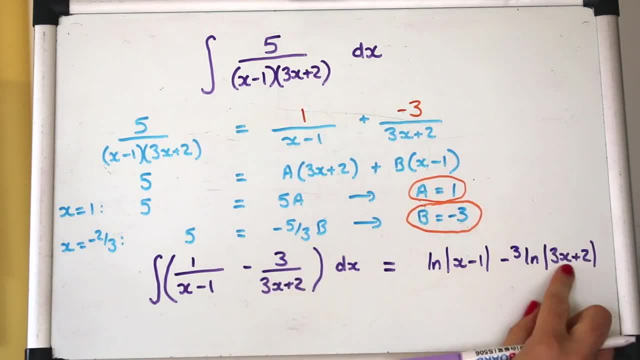 with the minus sign still there, The three on the top of that fraction can stay at the front there. but using the reverse chain rule on this, we would need to divide by the derivative of this function. So we'd need to divide by three. 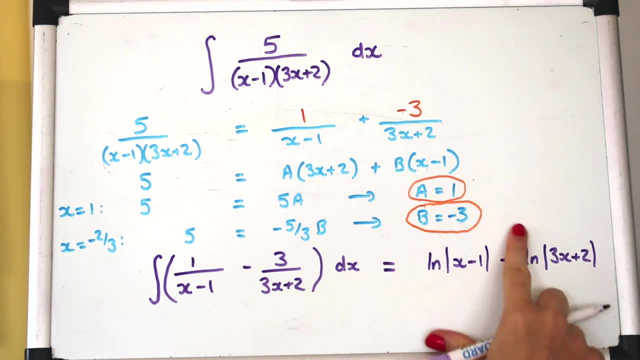 Actually that three divided by three at the front will just vanish. it cancels out. So that is that. And because it's indefinite, we must remember the plus c. So hopefully that's clear and shows you that the only way to integrate this is to split it up. 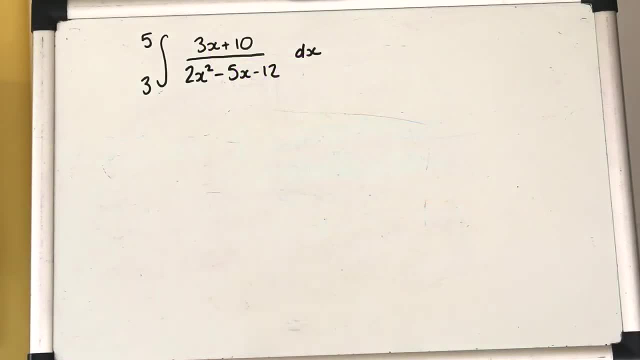 and then you can use logs to do it. Okay, this next question. just looking at this, it looks horrific, doesn't it? So, if you didn't know, we were doing a video on partial fractions integration. Think through how you might integrate that. Obviously, we've done a few ways of integrating. 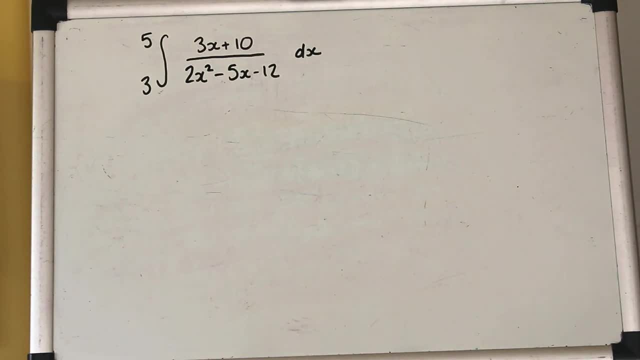 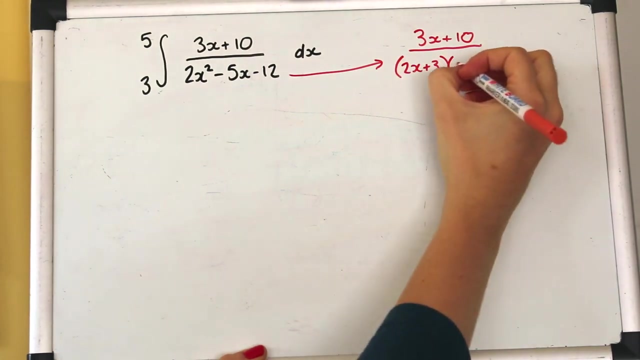 now. so you can run through the kind of checklist of how you can integrate something and that doesn't really fit any of them. But looking at what you can do, that bottom can factorize, so it's worth trying that. So factorizing that, putting it into double brackets any way that 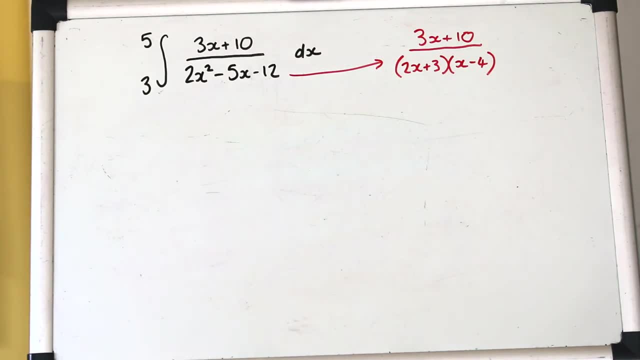 you're comfortable with. you can see that it looks like that And now that hopefully stops to look more like a partial fractions question, So we can try splitting that up. Same as last question, but this time I've just added some limits here, so we'll try a definite integration. 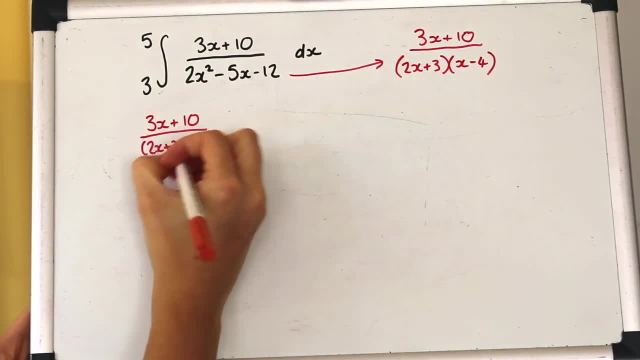 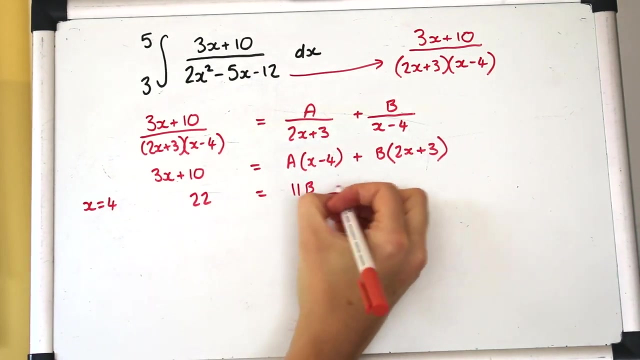 Do have a go at that. Okay, so partial fractions. here we go. Just to say I'm choosing values of x to force things to be zero because I found that easier. That is a horrible fraction and I did just pop that into the calculator to get the 11 over 2.. 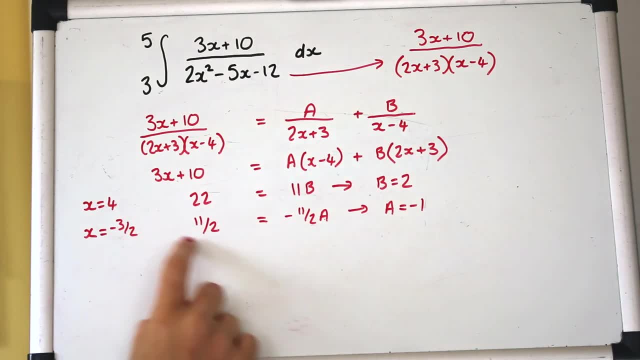 Okay, so putting that back into the original question. I'm going to rewrite this using the partial fractions. Okay, so I'm going to put that back into the original question. I'm going to rewrite this using the partial fractions, Using square brackets this time, because it's definite, and using limits. 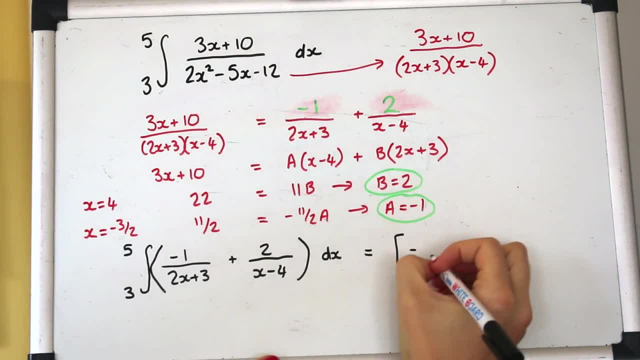 So here we've got a minus again. it's reverse chain rule, So it is a log, but we need to divide by the derivative of the inner function, so that would be 2.. So that can go up the front there minus a half. And then the next one is straightforward, because the derivative of 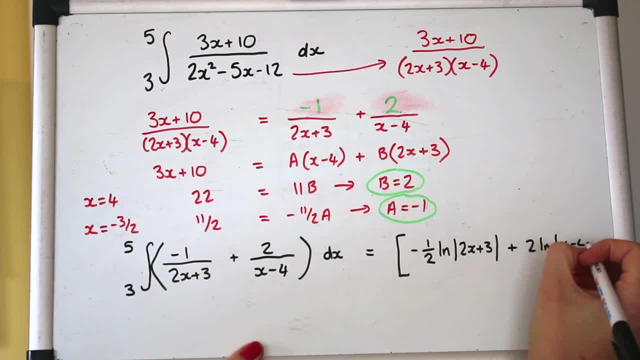 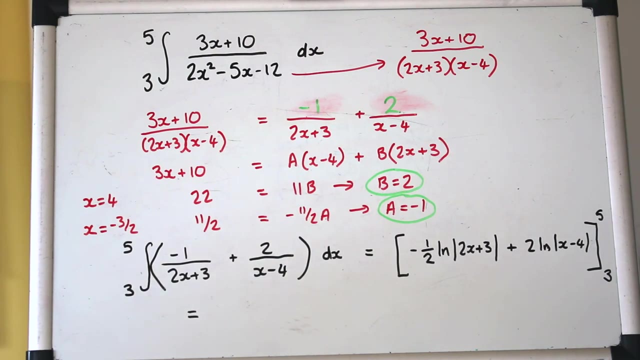 the middle function is 2.. So that's going to go up the front there minus a half. So that's just 1, so that can stay And the 2 will sit at the front there. Okay, when you put these limits in, sometimes an exam question will ask you for an exact. 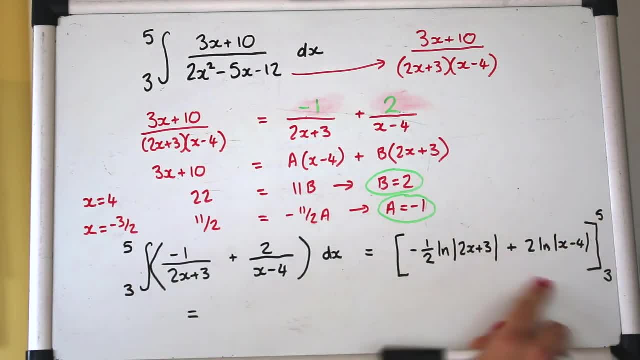 form as the answer. So if you just chuck that all into your calculator and get a numerical answer, that might not be quite what they're looking for- You can use it as a check, of course, but it might be worth breaking it up a little just to write it in exact form. 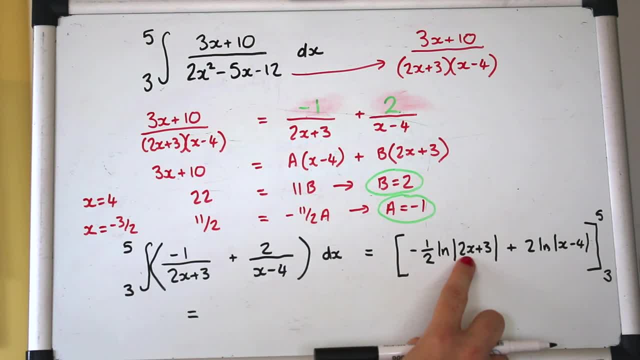 So we'll start with 5 in here. It will give us log of of 13.. I'm putting the 5 into here. 5 minus 4 is 1.. Log of 1, I hope you know is 0. So that would just cancel out that bit. So that's a 0. And then we'll take away. 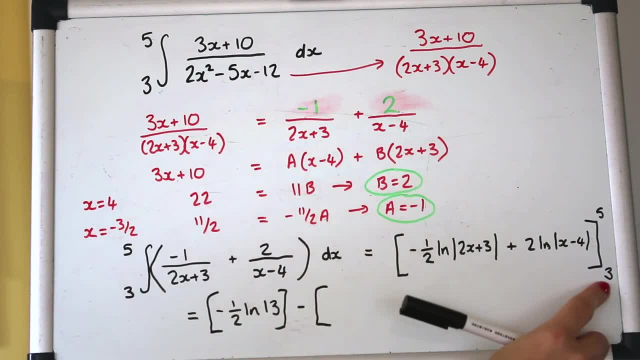 just keep that in a square bracket for now the second limit. So putting it in here 2 times 3 plus 3, so it's like 9, minus a half log of 9.. And then 3 minus 4,. 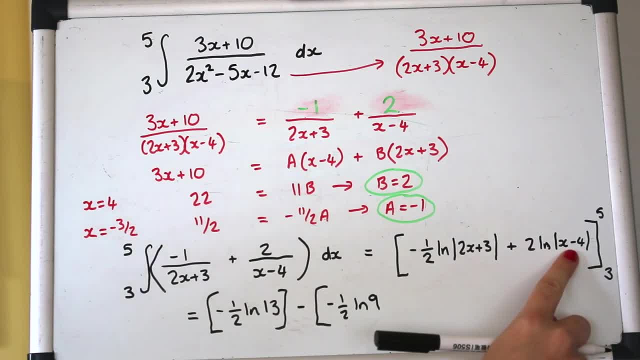 would give us minus 1.. We are applying a modulus to it so that would become log of positive 1.. So log of 1 again is 0, so that would vanish again. Love it when that happens. So we've got. we can tidy this up just a smidge. We've got minus a. 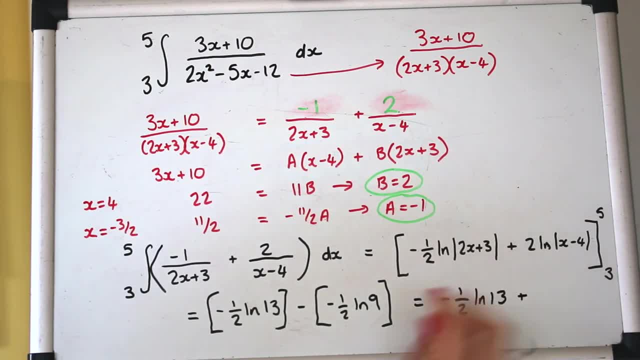 half ln of 13 plus, and then that log of 9,, we could bring that half up to be a power. So log of 9, to a, the power of half, and 9 to the power of a half is root 9, which is 3.. So you can. 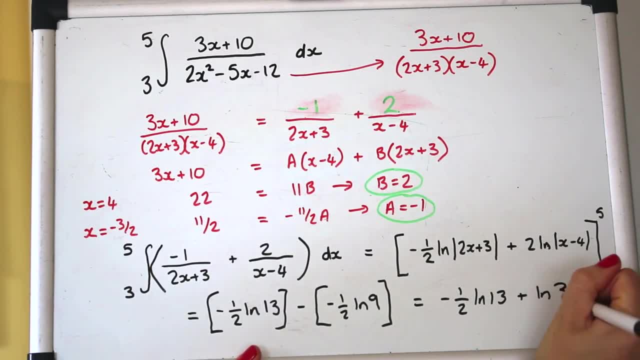 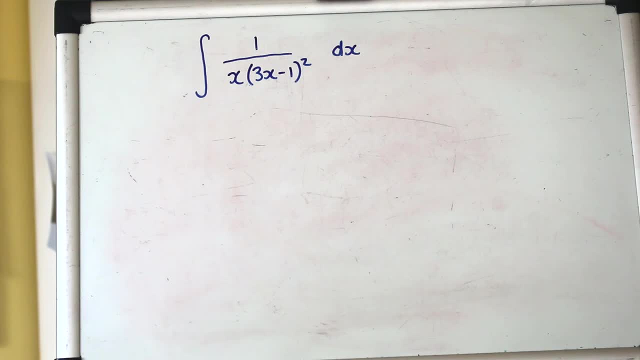 simplify that a little bit more Great, And we don't need a plus C because we've put limits in and that is that Okay. next question: I'm afraid that red pen has given my board a bit of a pink glow, but makes it more fun, I guess. Right, hopefully you can see again that this looks. like something we can split up. So we'll do that with partial fractions which isstraight from the course book that you'll give to me later, If I'm gonna be matching 123 to ID 3, which means that 3 has. 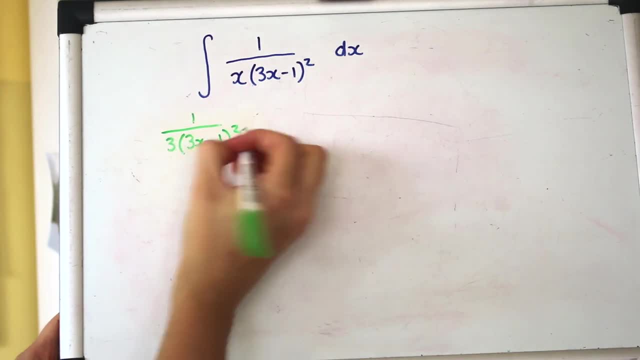 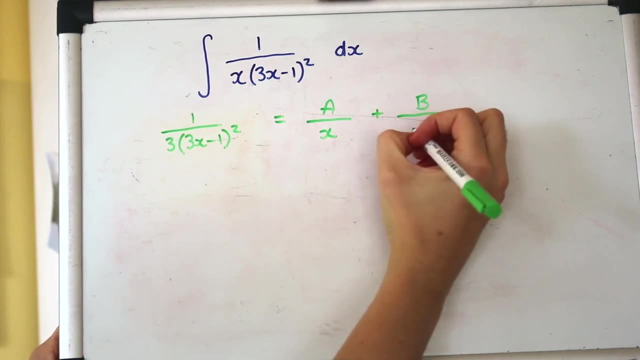 9 to the power of a half minus the power of a half, then root 9, which is 3.. So you can simplify that a little bit more. Based on that type of stuff once more. okay, this one's a little bit more complicated because it's got that. 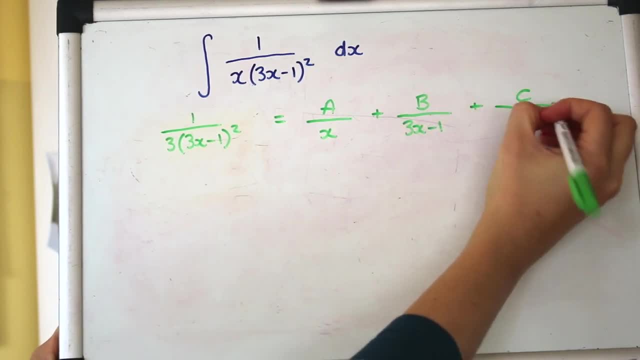 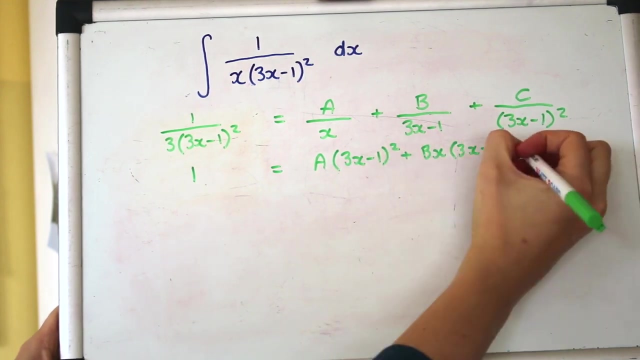 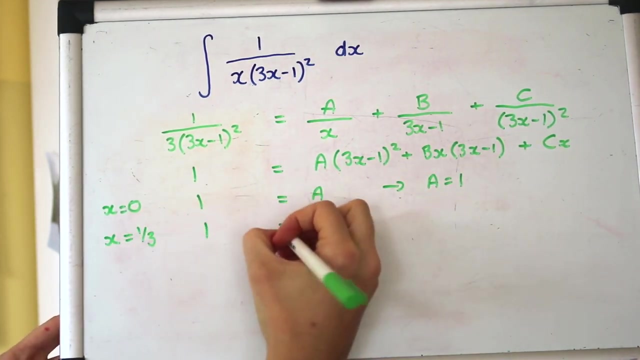 factor. so I hope you remember from your partial fractions that you need a factor of that 3x minus 1, but then you also need to include the factor when it's squared. so we'll have three different elements to this one. I've run out of things to make stuff serious or just pick another number out. 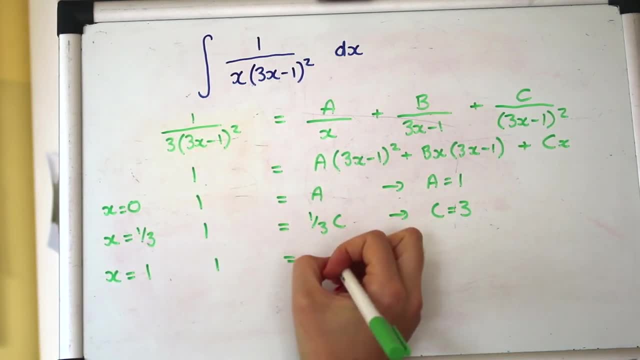 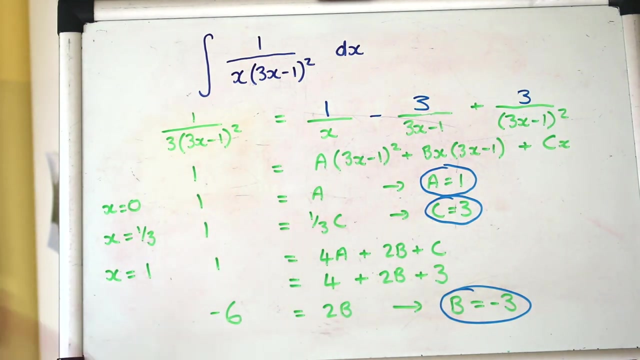 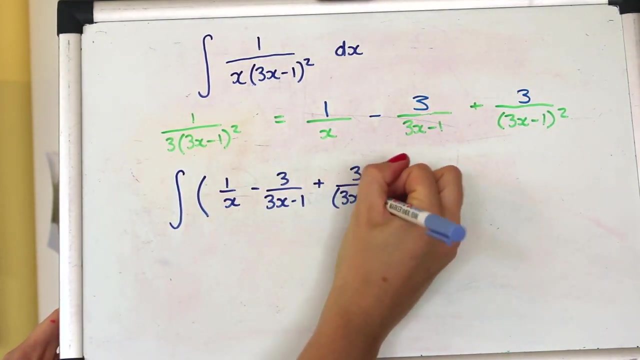 just go with one, okay. so that's the partial fractions bit done. I'm going to have to clear the board to give me some more space. okay, so we integrate like before now. this last one isn't a log, so just to throw that surprise at you and be aware of that one, because there's a power on. 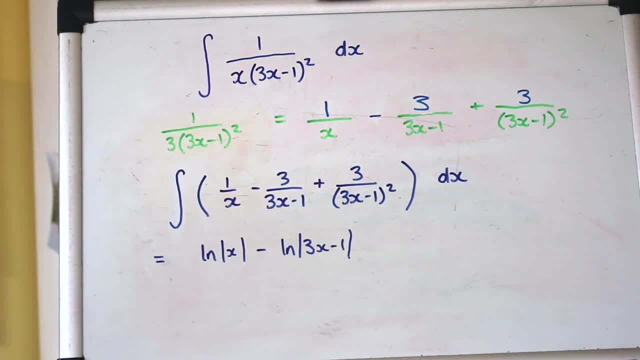 the bottom. this is a reverse chain rule so might help you to write the power at the top. so we've got 3x minus 1 to the power of negative 2, so we're integrating that. so we need to raise the power by 1 and then divide by. 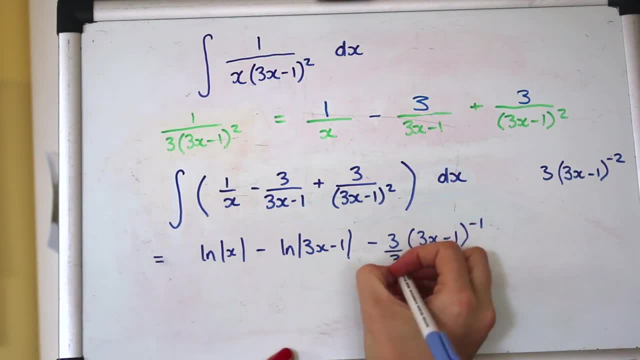 the derivative of the inner, which is 3. again, happily that cancels the 3 at the front out, so that just vanishes and that's the final answer. you can write that back down at the bottom. so 1 over 3x minus 1, if you want to, and again we've. 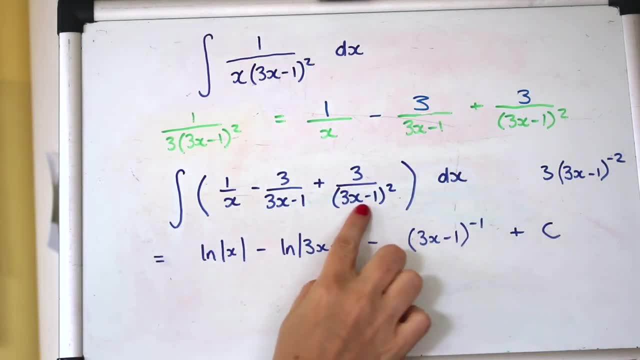 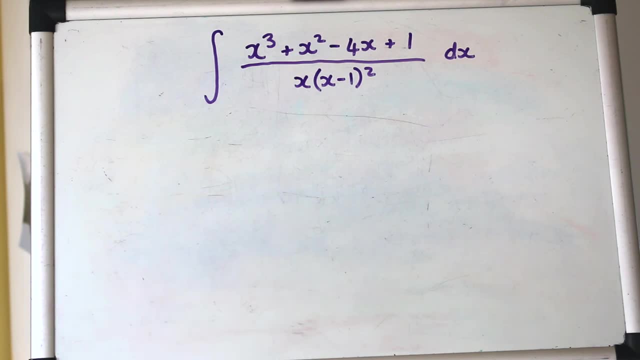 gotta plus see, because there's no limit. so do watch out for that. that's a bit sneaky. well done if you got there right, okay, last question, and this is an absolute beast that I made up for you, you're welcome. so it's another partial fractions question, but can you spot what's harder about this one just before? 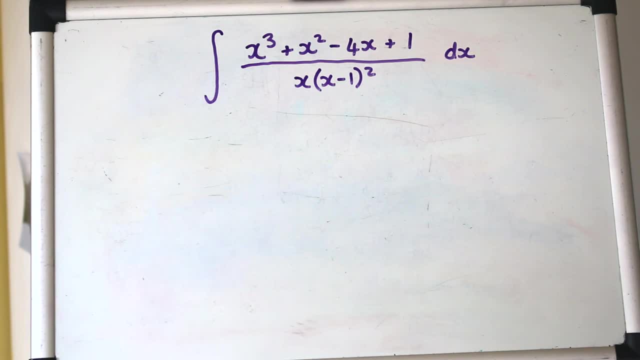 we begin this one to get one this hard. but you know, if you can manage this, you can manage anything, so let's try. so the bottom: if you expand that out, then the highest power of x would be cubed. notice that we've got an x cubed on the top so we don't have a smaller numerator than denominator. they're the. 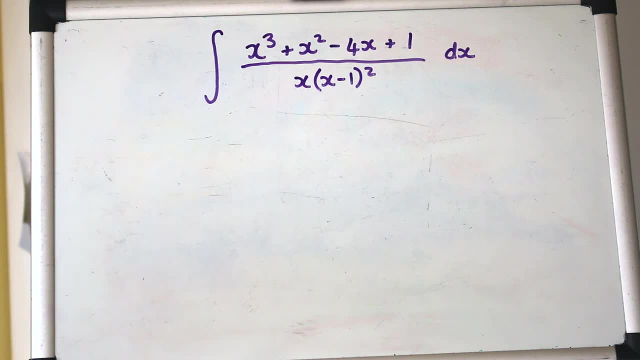 same, and what that suggests is you can pull out a number before the partial fraction, so there's going to be a whole number to start with. again, this is in my partial fractions video, so just be aware of that and practice that, and I showed you a little trick: how to pull out the number at. 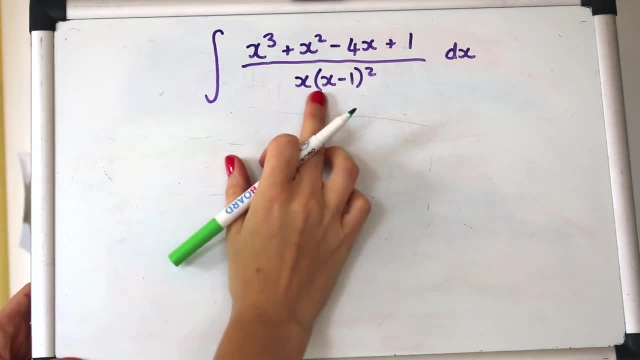 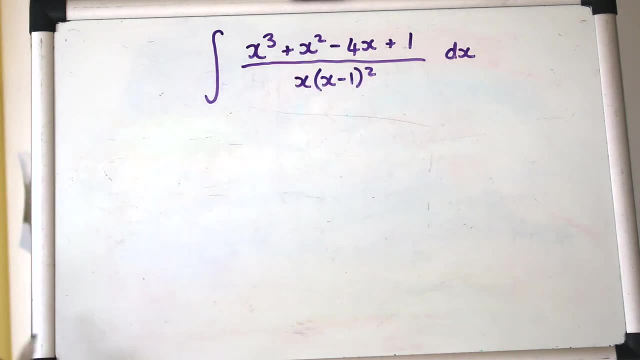 the front. I'll show you now. so what I mean is, if we expand this denominator out, then we could get a multiple of that on the top. so that's what we're looking for. first of all, let's expand that denominator. if we expand out double brackets- x minus one times x minus one- 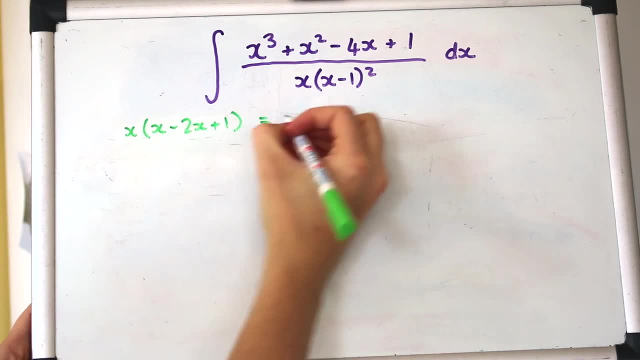 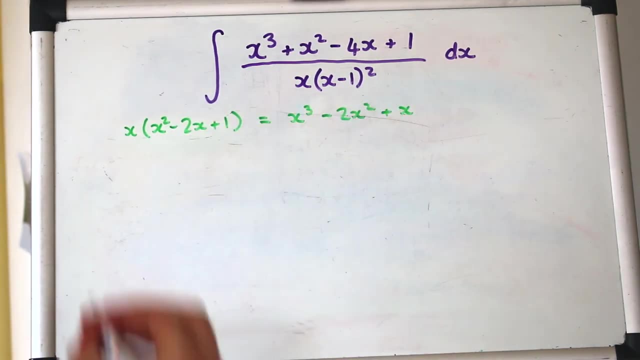 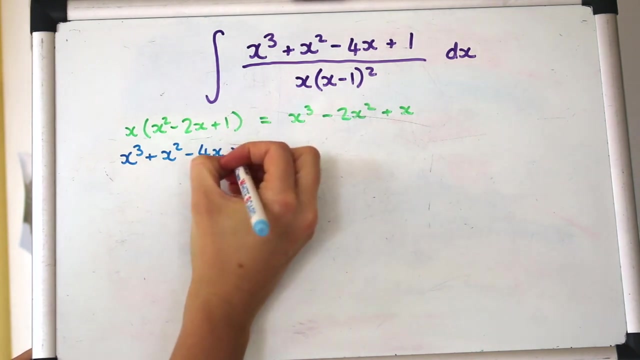 first of all, and we'll get that, and then we can expand by the x, and then what we want to do is write the numerator in terms of that. so we're gonna rewrite that first and we want a number of these with other things: x cubed and x cubed. it will only be one of them if there was a two. 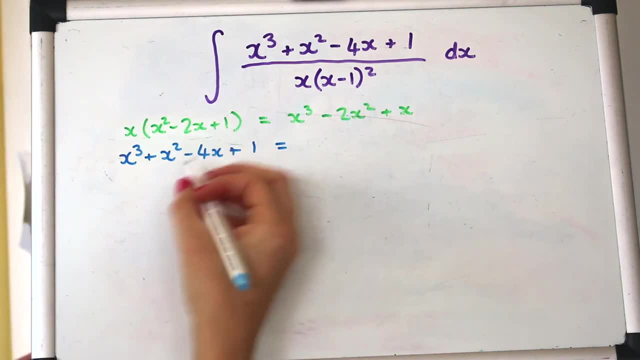 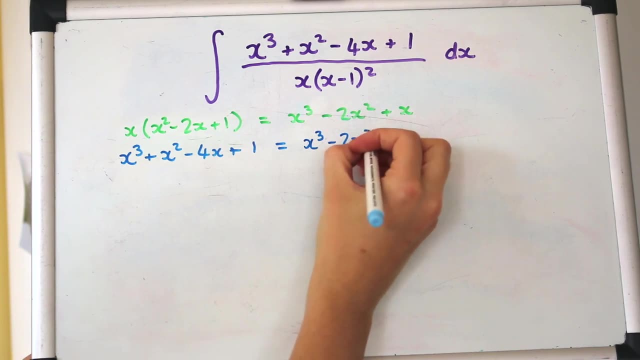 in front. then you could do two lots of all of it, but it's not, so just one, so one lot of all of that. we'll just write that out again. so we're gonna have one lot of that. but then we need to adjust. we've got x cubed which agrees. that's great. but 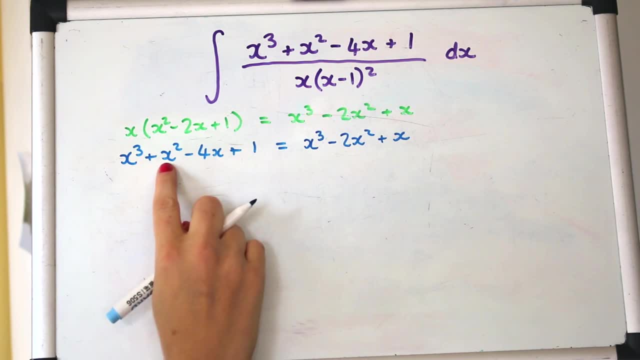 we don't have minus 2x squared. what we want is plus 1x squared, so we need to plus another 3x squared to make that right. we don't have X, we've actually got minus 4x, so we need to take off. 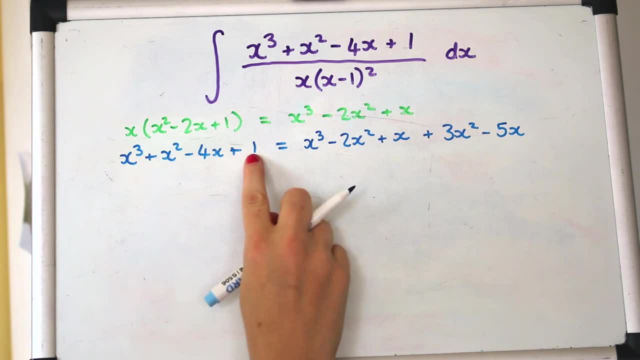 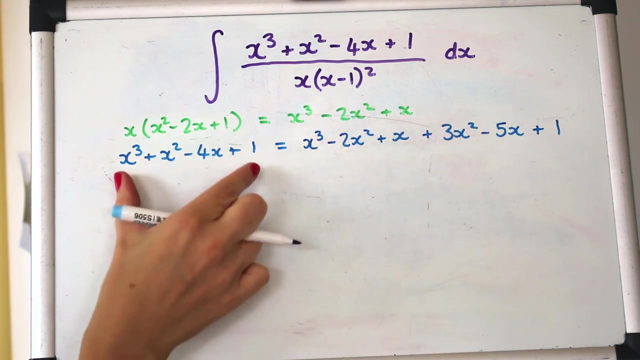 x and we also need a plus 1. so can you see, I've written that in terms of that denominator, but then if you collect all this together, it does agree with the left-hand side. so just to make that even clearer, I'm just going to write the denominator on both sides. 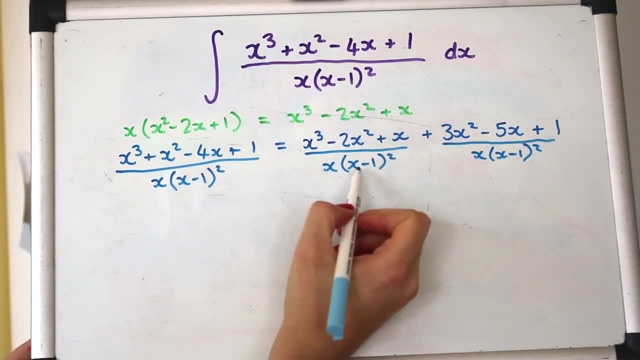 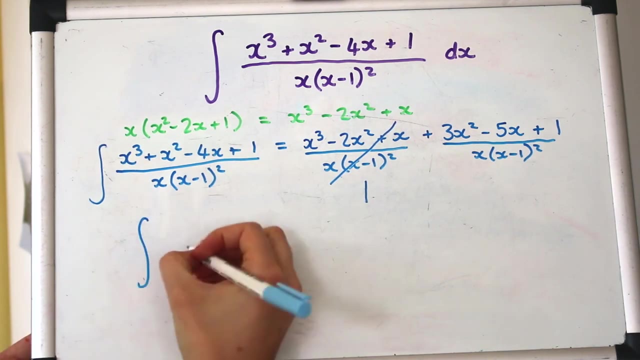 so that top is the same as that, so that all will cancel out to just be 1. so if we're integrating all this, then we can rewrite that as the integral of 1 plus all that jazz there. so we are integrating 1 plus this stuff and that's the stuff that we can now split into partial fractions. 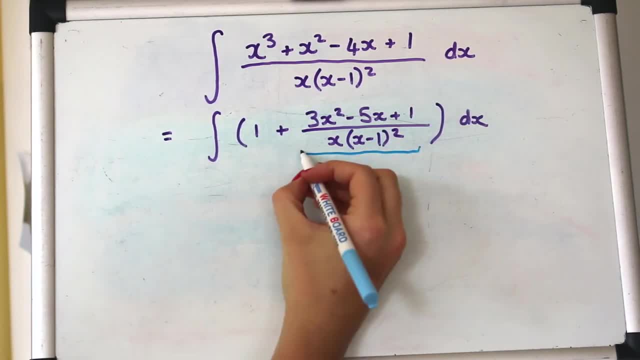 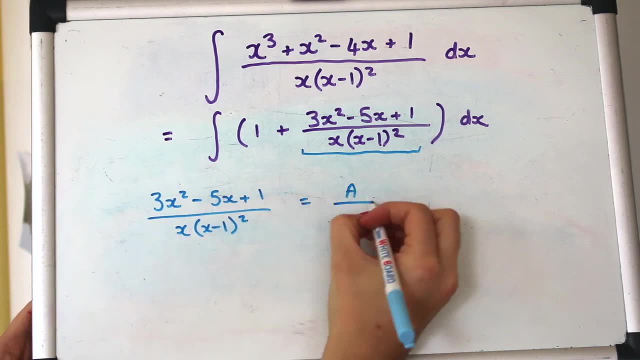 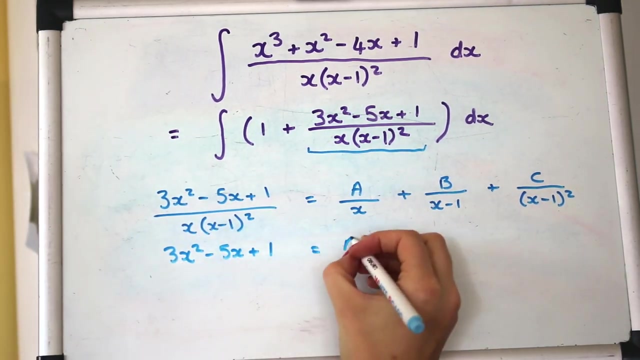 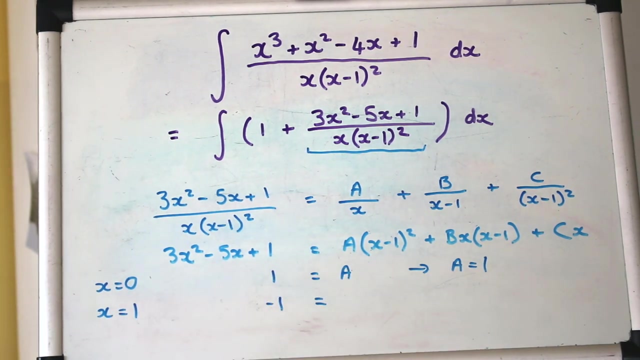 okay, so we're now just going to take this bit here and split it into partial fractions and just be aware, this is another one where you've got that factor repeated, kind of one with a squared one, not. so let's try that now and this next one. 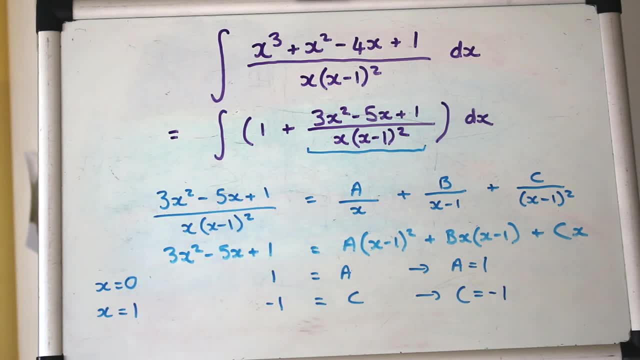 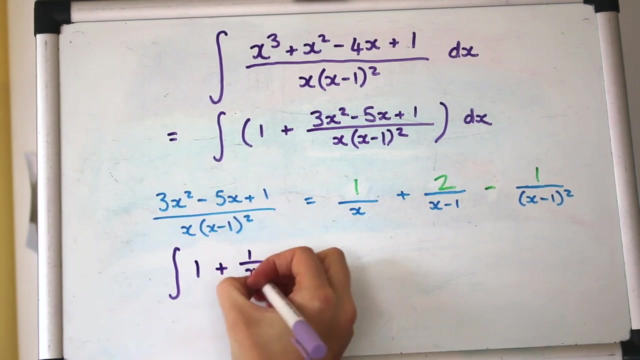 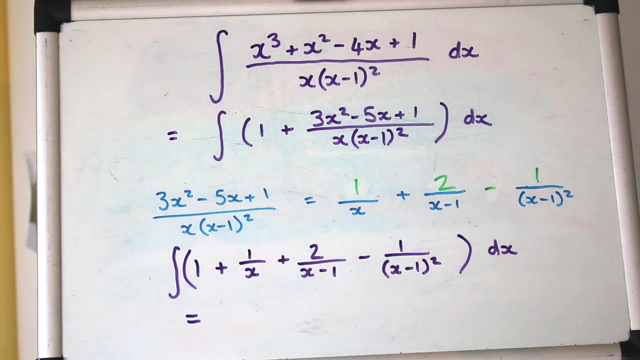 one goes to 1 squared fear and fifth square and second square meter square, 8x square plus precise 0x 3x. Okay, so now we can write the integral with all that simplified And hopefully we can now integrate that. That last one- just beware, it's not a log, because it's got a power on the denominator.